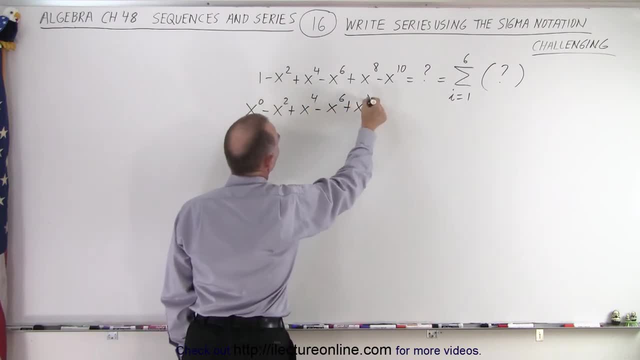 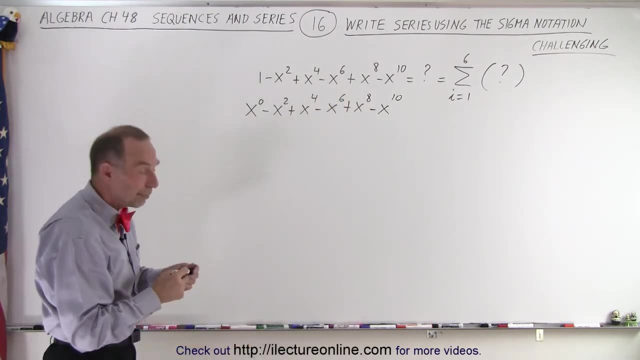 to the fourth, power minus x to the sixth, plus x to the eighth, minus x to the tenth. That's exactly the same what I had when I started, but now you can see a little bit more uniformity between all of the terms. All right, now notice. 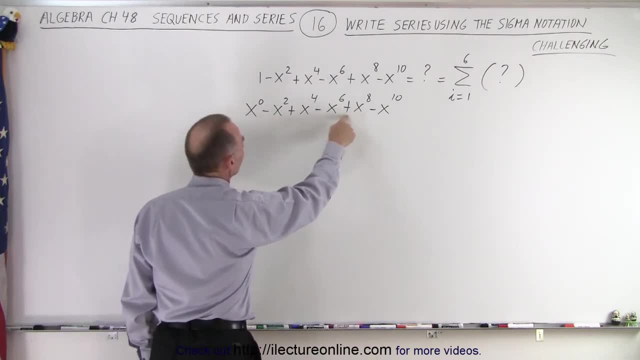 the signs also alternate. I have a negative, a plus, a negative, a plus, and the exponents increase by two, even though i increases by one. So if I go two times i, that makes it increase by two. So I believe that I can write this as follows: This is equal to this sum from i equals one to six. 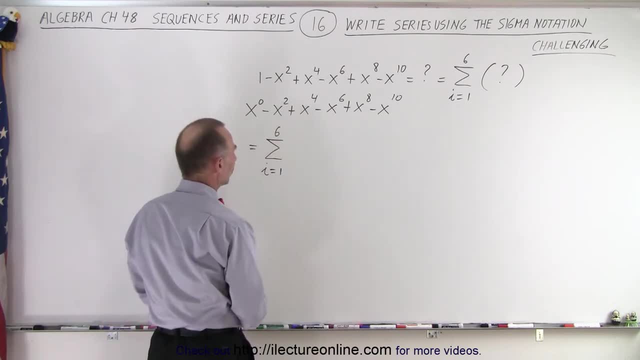 We already know that we started one and we end up with the number of terms. We need to take care of the sign, and the first sign is positive. So how about this? The number negative one raised to the i plus one power. So when i is one, the exponent. 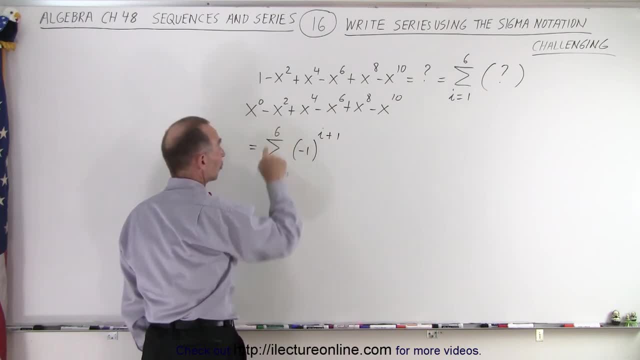 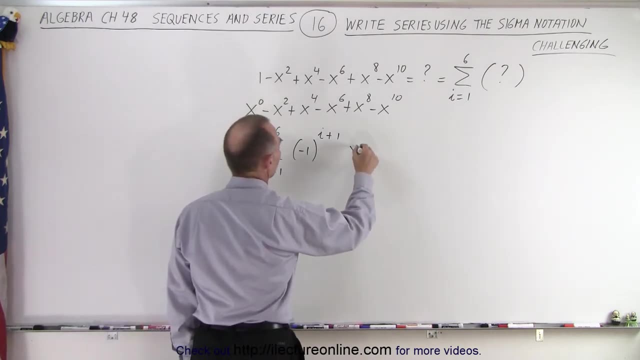 is two and it becomes positive. When i is two for the second term, I get three the exponent- I get a negative. So that takes care of the sign. Now I need an x. Raise some exponent and notice I need. 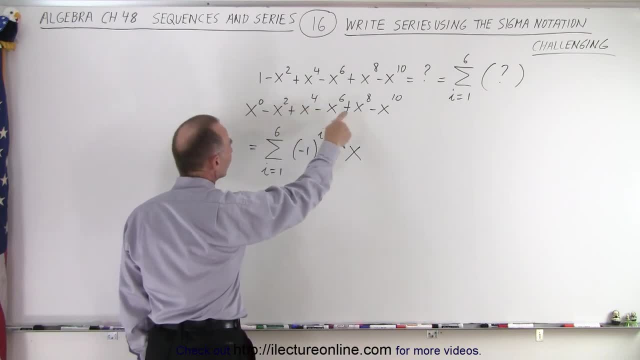 to have two times i because I need to go from two to four to six, to eight. Well, it's actually starting at zero, So I need a two i there because I need to increase by two When i increases by one. 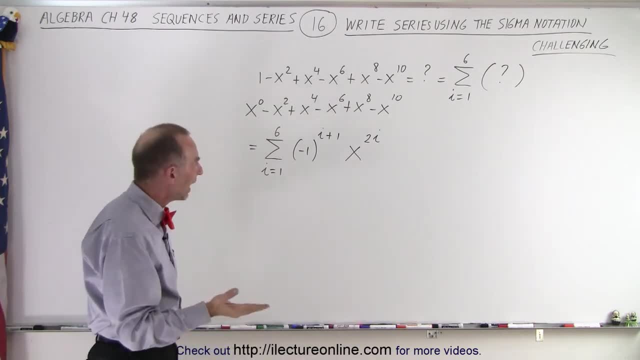 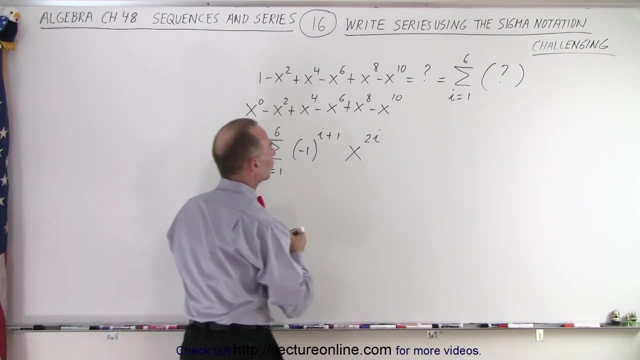 I want the exponent to increase by two, but I need to start at zero. And when I plug in the first value for i and get two times one, which is two. but since I want a zero exponent, I need to subtract two to bring the first exponent to zero and then everything else after, that will work. 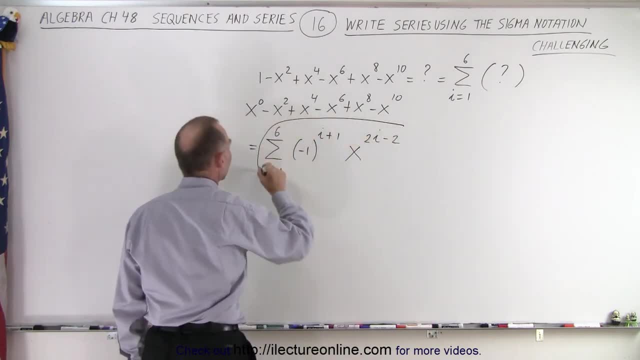 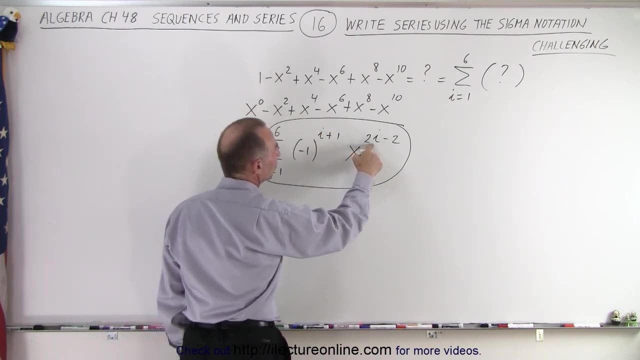 So it looks like this is a proper way of writing this in a summation notation. This will give me the correct signs. This will give me the correct change in the exponents. for each increase in i, It increases by two, but I need to start at zero, so I need to subtract two to give.